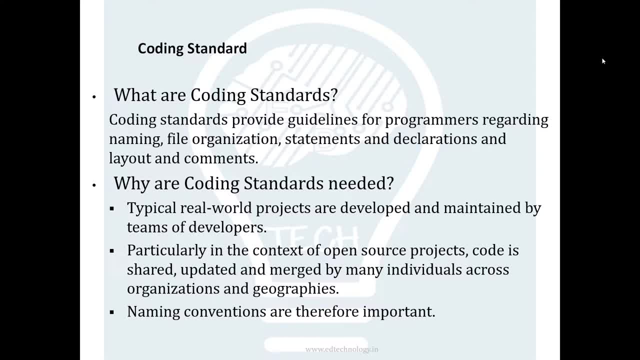 It includes the naming of the files, the file organization, the statements, the comments and so many more things we will be seeing in the further part of the video. Also, it is very important for all of you to understand why coding standards are needed. See, if you see the example of the code which you are having in your project, there are multiple people working and sometimes, though, you guys are working in the same location together, it becomes very tough for you to understand what that particular code is coded by a team member. 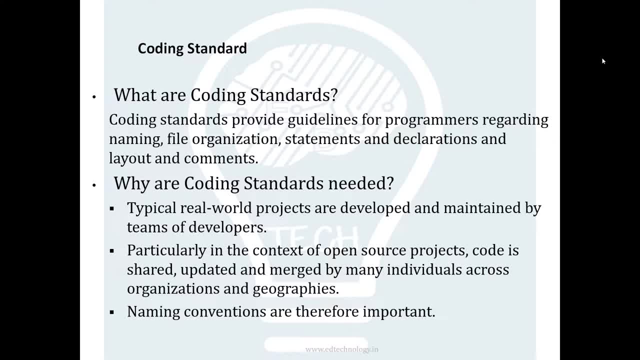 But in a typical real world this becomes even more worse because there is a huge team of developers. Sometimes they are geographically divided and from different places. Since you are not following the same standard of the mechanism, it can become very tough for others to understand the code. 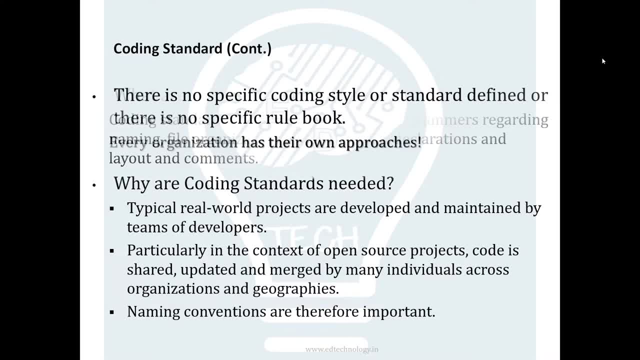 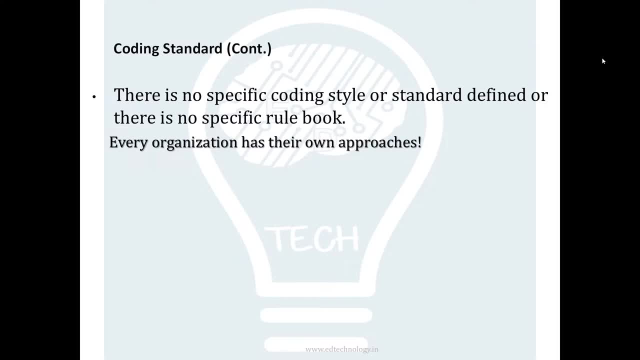 So that is why the coding standards are. you know, if we were to understand company-wise- a lot of people ask this question while I'm teaching the subject- that what is the right standard or what should we follow? Basically, there are no specific coding standards. 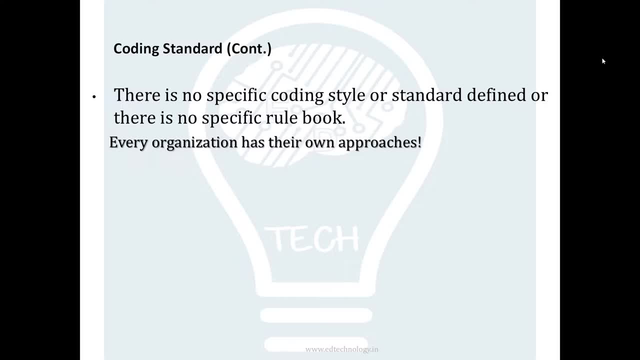 There is no standard defined for the you know coding. There is nothing as in the specific rule book, because every organization follows their own approaches. They have their own styles, In fact, within the organization. so the overall umbrella is the same within the organization. 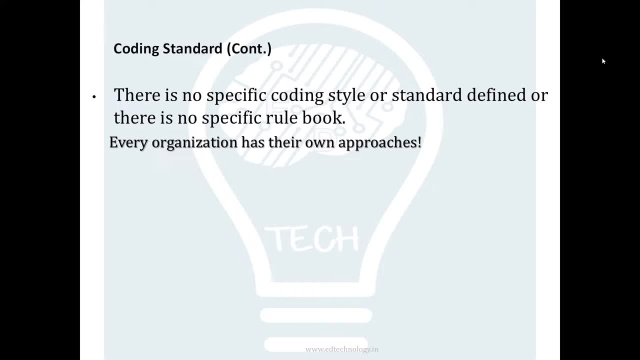 Teams also come up with their own approaches, So that once you start working in the companies, you will come to know. But there are certain things which are very common in each of them. So, like you know, first of all, yes, 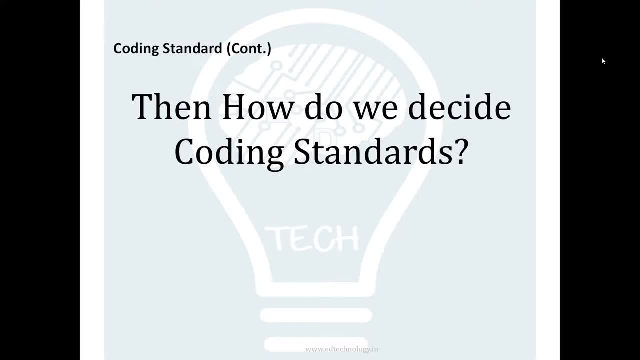 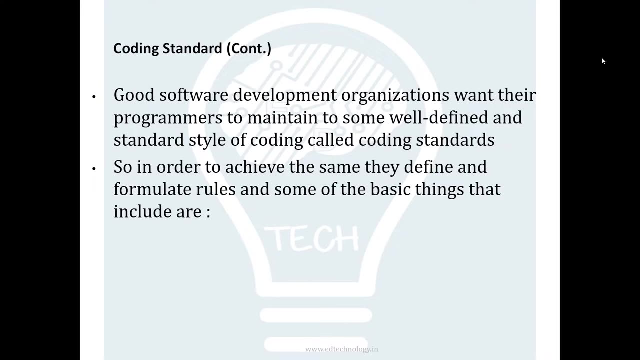 Question arises: how do we decide the coding standard? A lot of people, a lot of very good students in the classes, ask me: what do I follow to achieve a good coding standard? So a good software development organization wants their programmers to maintain well-defined standards and coding styles. you know where it is having a few things. 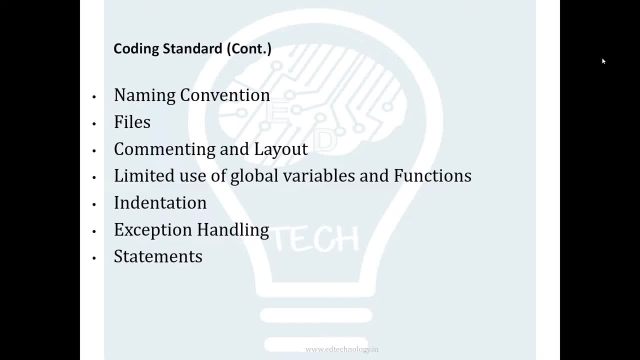 Those few things include this: The naming conventions for the variables and the files. How do you organize the files? The layout and the configuration, The commanding and the documentation part. Usage of global variables should be minimal and also even global functions should not be used much. 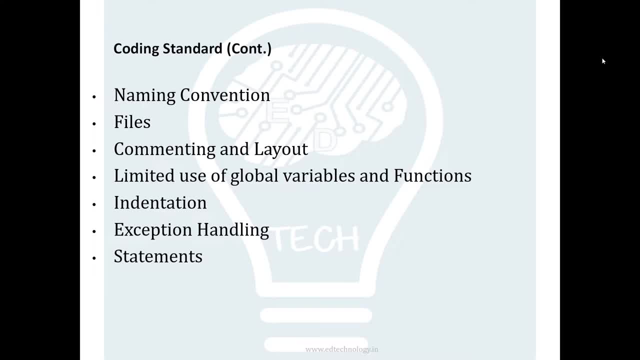 Write set of indentations. so you understand how the code is organized. A very good exception handling. In fact, the worst part in the coding when the newbies are doing is poor exception handling. You have to pre-plan and think about the possible errors and you have to come up with exceptions for them to be handled well. 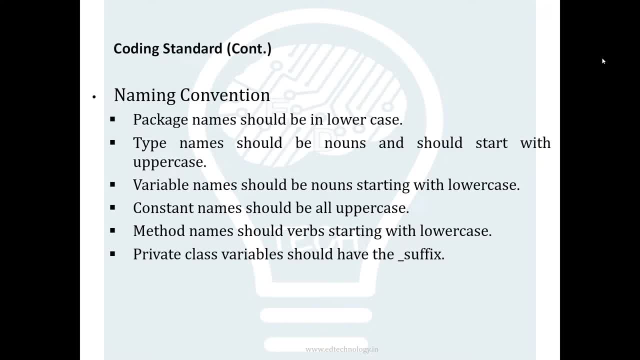 And the statements, So let us see a little bit of detail in here. So, basically, naming convention must include few things that your packages- and this applies mostly to object oriented, though some of the things will apply in different languages also- And now if you see NET, Python, Java, all of them use the object oriented methods. 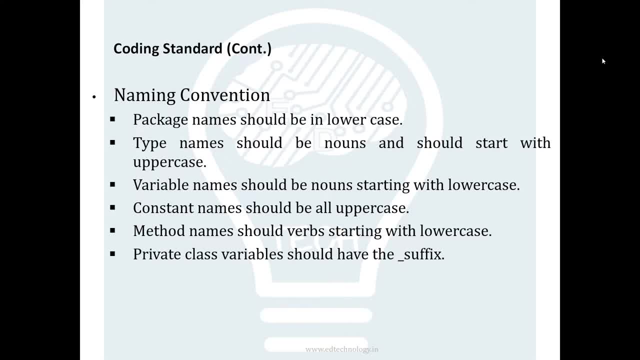 So we have to understand that. So packages have to be named in lower cases. The types of names should be nouns. It should start with uppercase So you realize that you know type names are specified in this way. Variable names again should be nouns and again it should be in lower cases and it should have constants all in the uppercase. 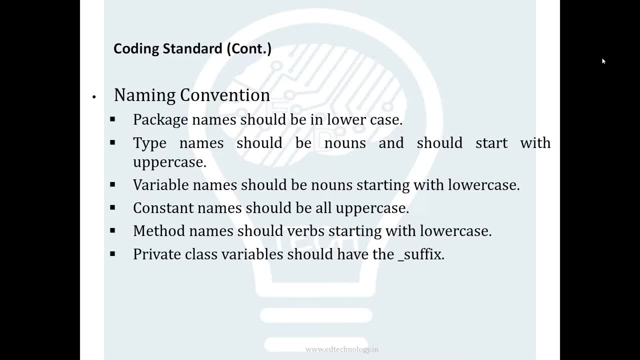 So we realize. So these are the simple mechanisms we follow in the code. So, seeing the variable and other part, we can find out what is a variable, what is a constant, where the methods are and similarly the code: debugging or upgrading. 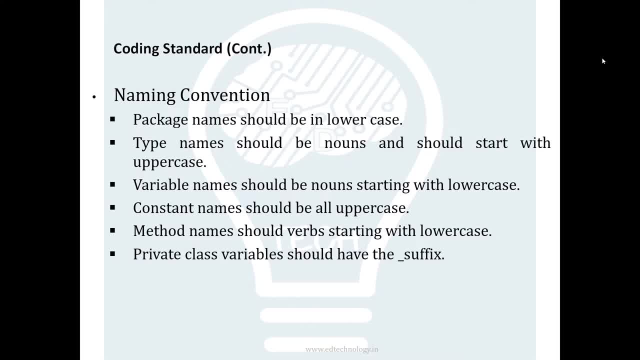 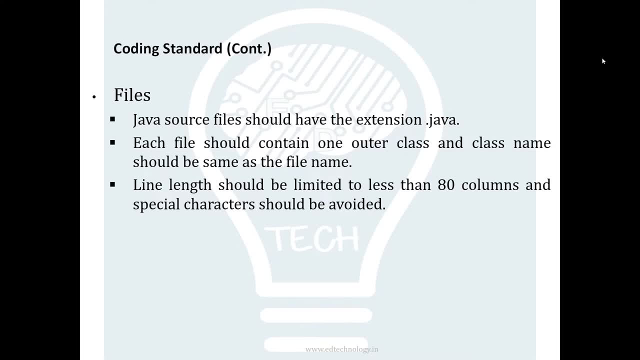 And similarly the code, debugging or upgrading. But when parallel coding happens, it becomes better. Next thing you understand is that files- each of the files- should contain auto class and class be named as the file name and class and the class name should be named as the file name. 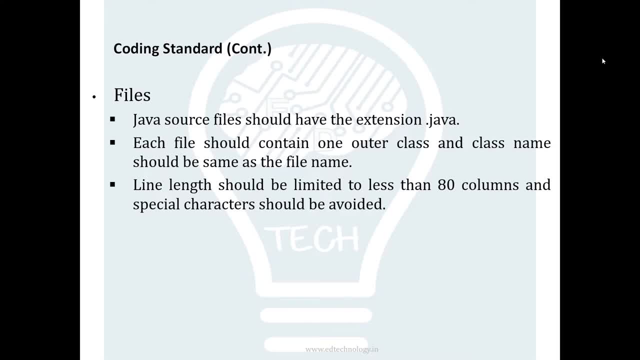 So otherwise what happens is with coding multiple files in the project, and this will happen Once you start coding for final projects or projects which are doing an internship and the training. Then you have to realize that there are multiple files there And if you are not naming them properly, 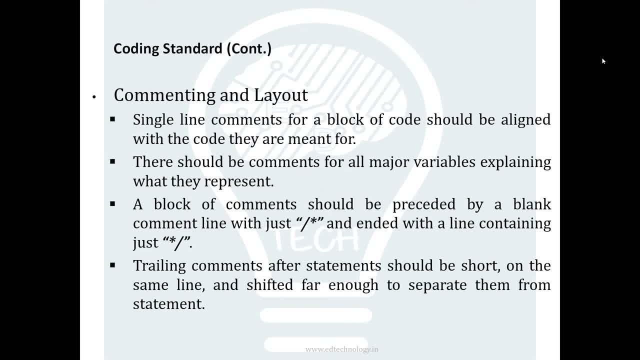 you will land up with the problems then commenting a layout, a very important part in the coding which would have learned in the initial part of the university syllabus where the programming was taught. but people do tend to forget that part that we have to give appropriate comments, you know. 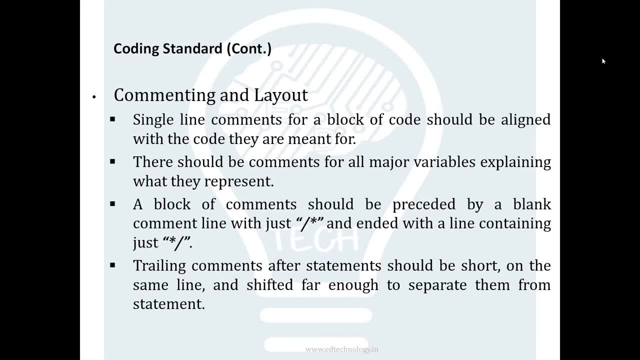 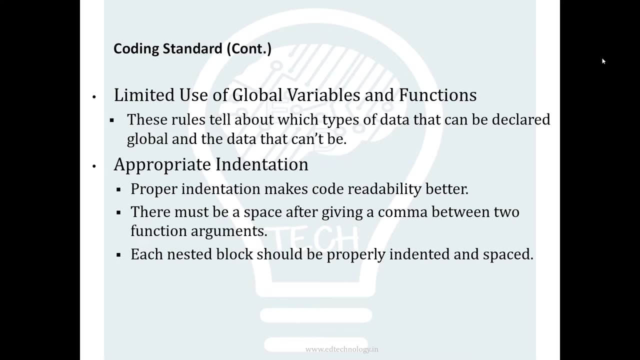 preceded in a lot of ways and those comments define where and what code is. so you have to understand how those codes work and how the commenting and everything is aligned- very important. what which the naive programmers forget is where you know they use lot of global variables and functions. in fact, even in 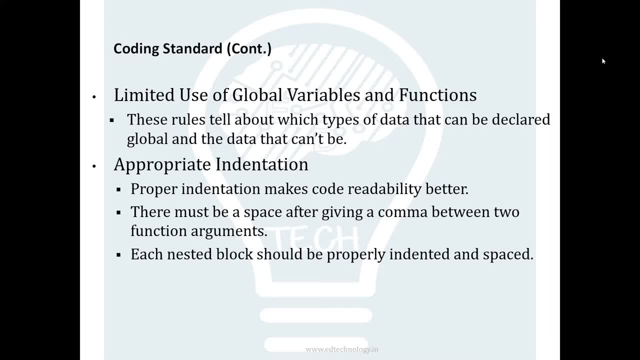 the editor files, which is to be discussed further- they keep everything in the global files. and then, because they want to avoid the errors of you know where function is not getting a value or variables are not reached, but it may lead to lot, of, lot of security bugs. 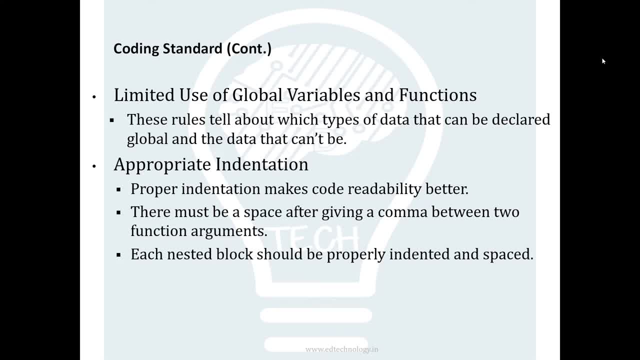 so please avoid that. use appropriate indentation, because the readability is better, so the debugging is better, and also starting of the ending of the functions. if you are using dotnet, dotnet does it very well by itself, the editor itself, but if you are using languages like Python or C++, it turns out to be 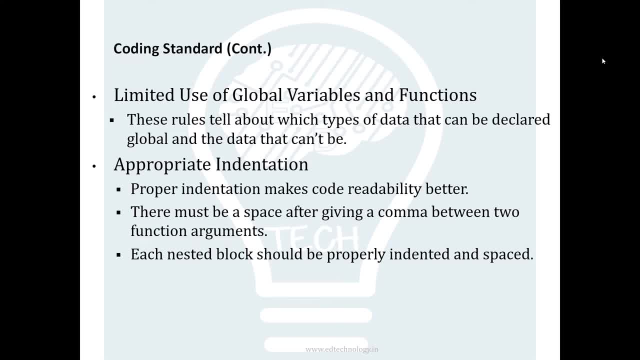 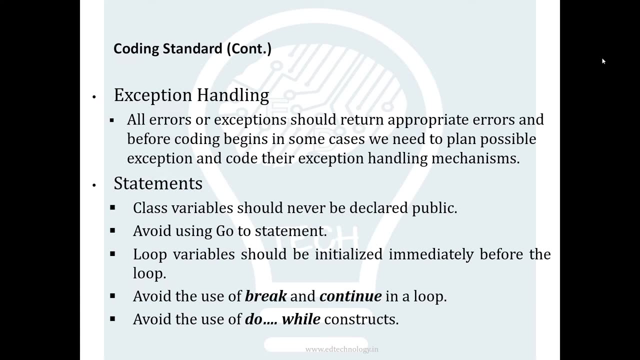 the programmer who has to do the most of the work. again, if you are doing Java, there are editors who does the indentation well by itself, but you are doing it in a cool way. please make sure you are following that practice. exception handling: i told you in the earlier part of the video itself. it is not planned well. you are not knowing what. 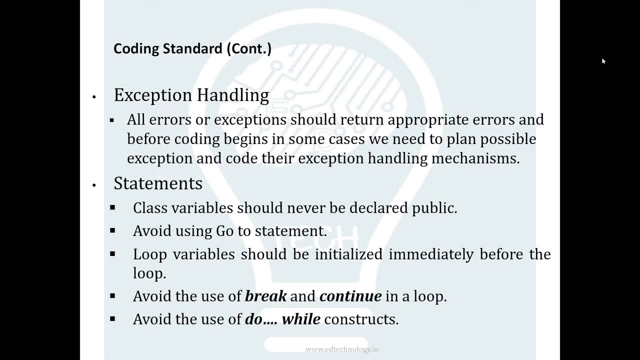 errors should be given and ultimately, when a user is using it, they do not understand what mistake they are committing. so if you are not having exception handling, or even while somebody is coding, they do not understand what is going wrong. so you need to have appropriate error mechanisms. 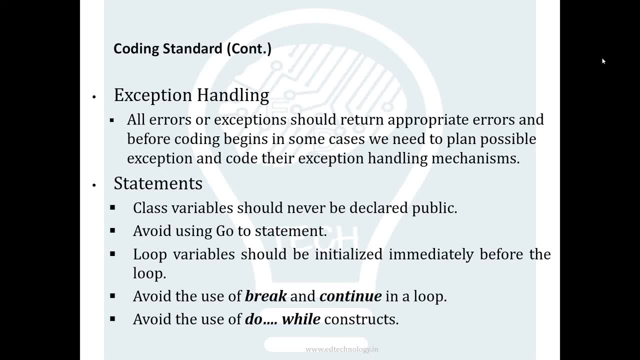 and exception handling, while coding itself is part of coding standards and this is, if you do not follow, ultimately in a large project, could lead up to a lot of errors. statements so uh, you know, i'll give you a simplest of example. avoid using go to statement, this kind of up and down logic. 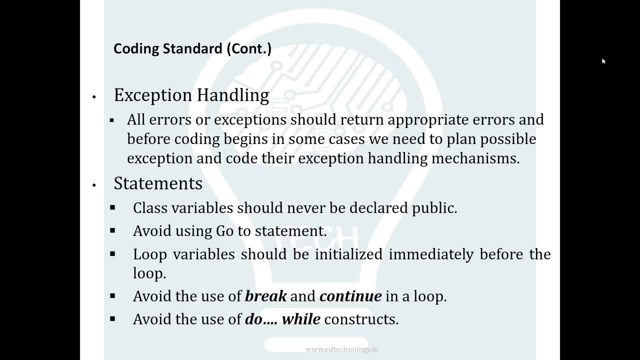 which you have done in the. you know simpler languages like c would not work when you're doing a project. so whatever standards you are talking about in here i'm related to the project coding, or the coding as in part of the software, project management. so please understand those kind of statements can lead up to a lot of errors in there, so this: